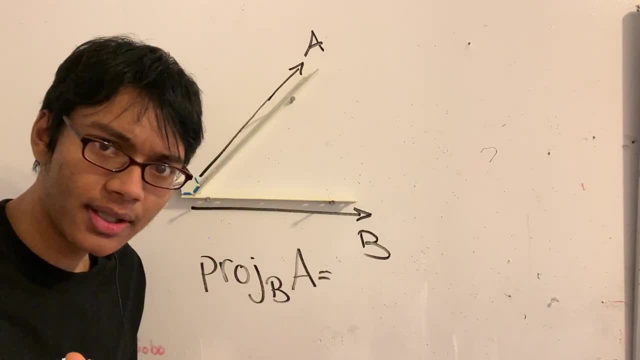 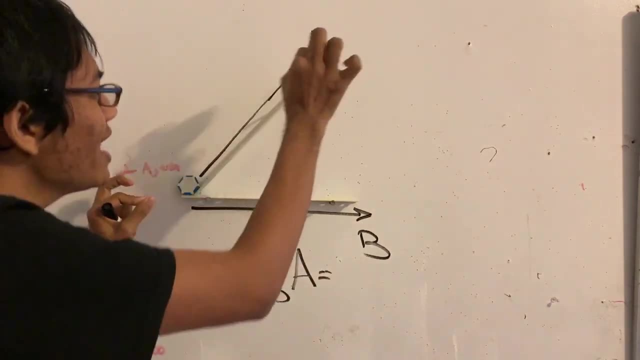 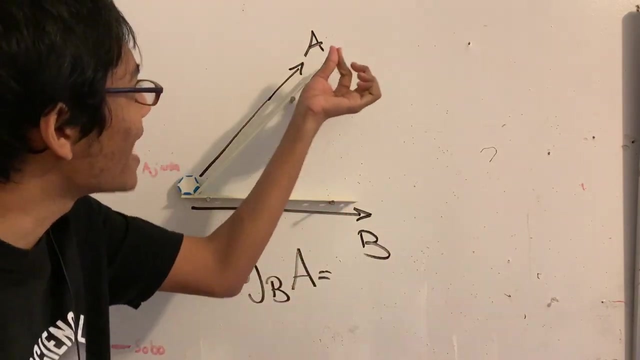 what do we actually mean when we say projection? You see, when I say I want to find the projection of a onto b, I mean how much of vector a is going in the direction of vector b. But here's another way to think of it. Imagine there was a street lamp on top of vector a. 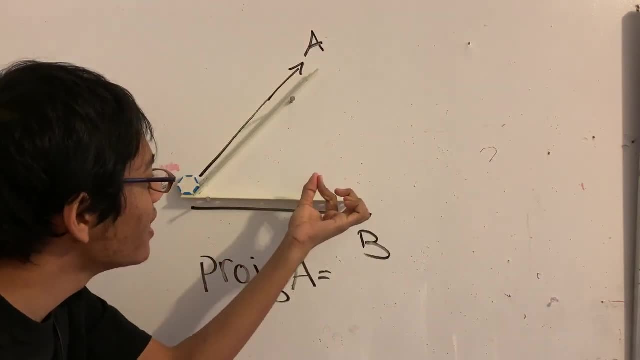 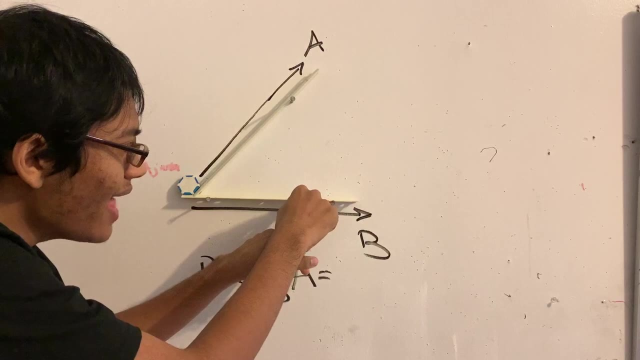 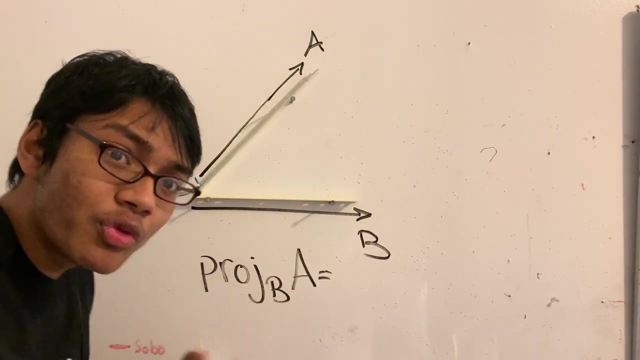 and it was shining down on vector a. Well, it would shine down in just the right way, so that a bit of the light would pop up here and that bit of the light would go on top of it. light would be the shadow of this vector a onto vector b. so when we say projection, we're really 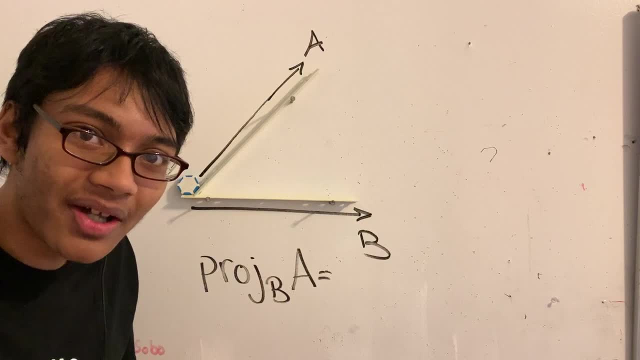 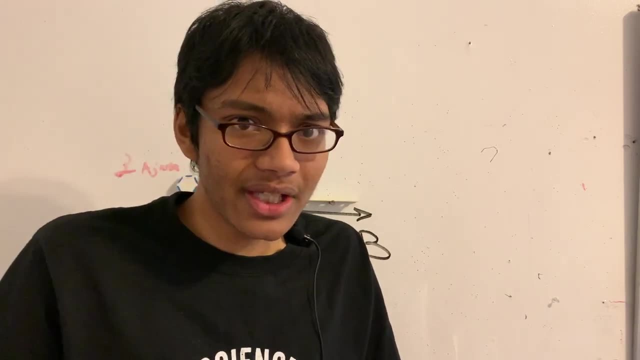 talking about shadows, but you don't have to think about it, you don't have to imagine it. here it is. this is a 100 milliwatt laser classified as a weapon here in the us, but today we're only using it for educational purposes, if i screw off the lid over here. 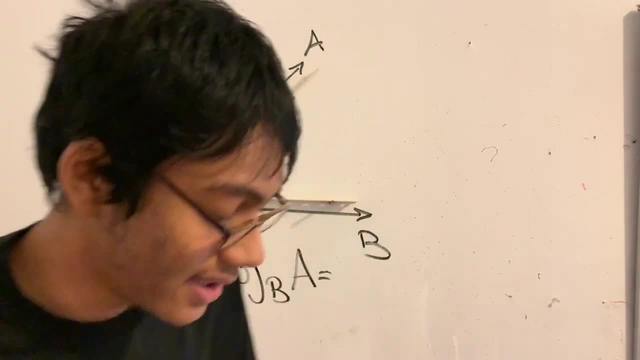 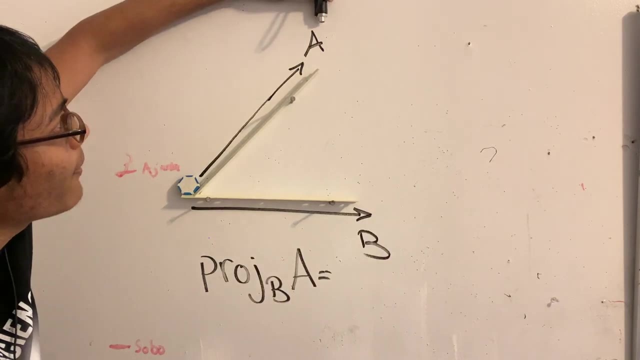 so that the light is not too focused, otherwise it would be blinding. then i can shine it from above, vector a, almost like a street lamp right, and what do you think is going to happen? what's going to happen? well, what's going to happen is the projection, the shadow of vector a is going. 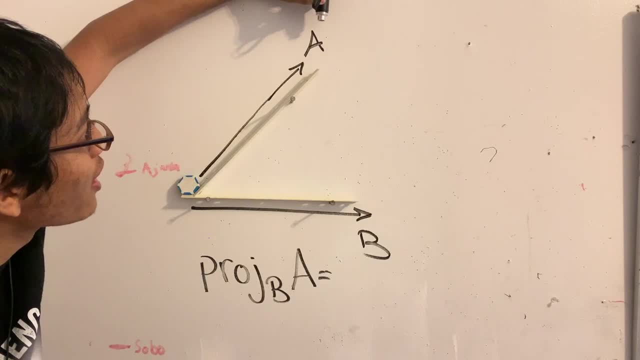 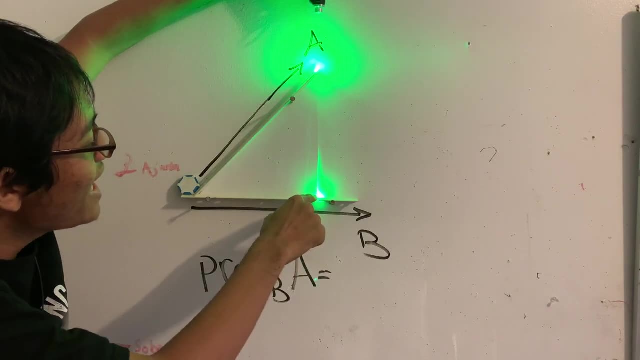 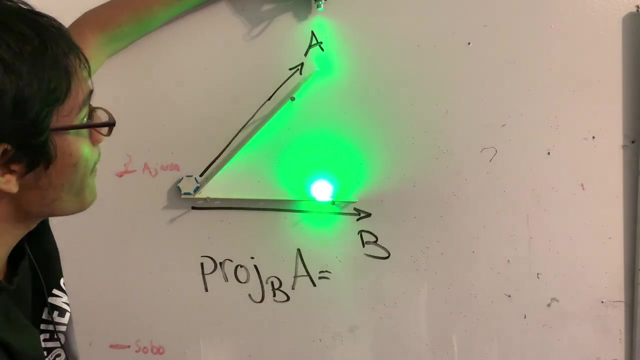 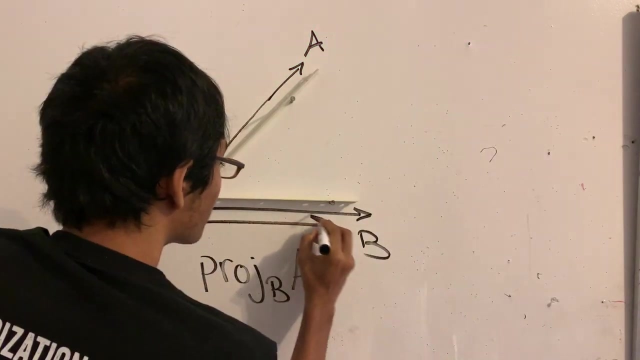 to pop up on vector b. let's check it out. enough talk and there you go, that right, there is the projection of vector a onto vector b. now look at that closely and you'll realize something of major importance. right, this projection is a vector. that projection itself was a vector. right, this was the projection we were looking for. 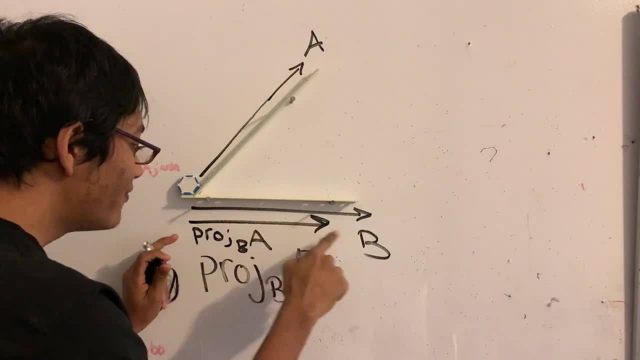 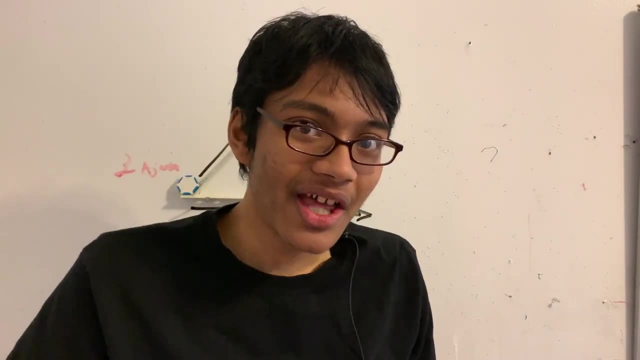 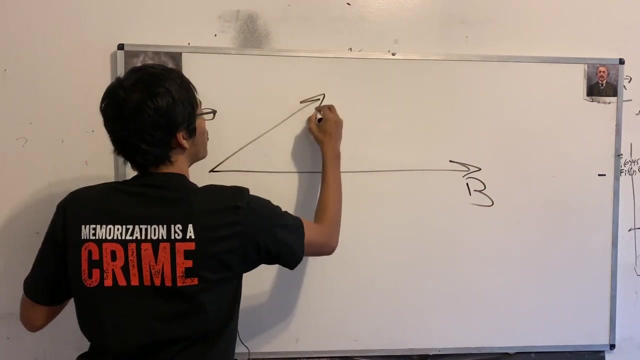 praj b a, and just like any vector, this projection has a magnitude and a direction. but how do we find that magnitude and direction? that's what we're gonna do, all right, so here's the deal. i got my vector b right here and my vector a right here. of course, i want to find the projection of my 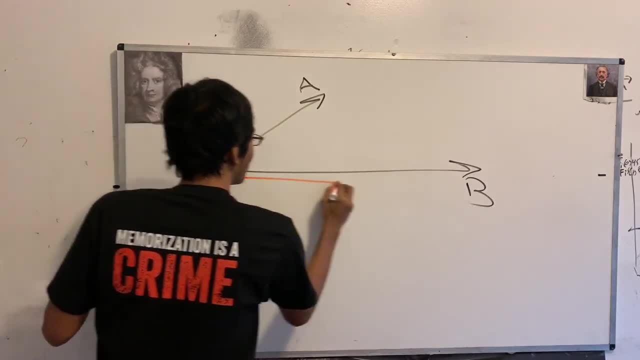 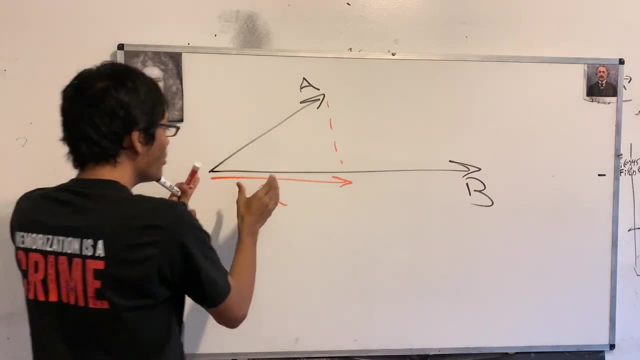 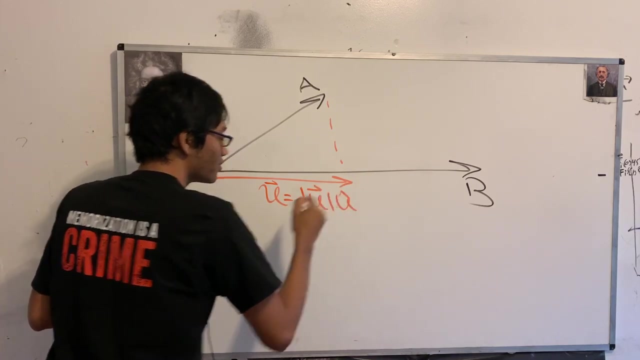 vector a onto b, which is going to look something like this: this vector, this vector, let's call my projection vector. you, just for the time being, now, now, now, now. how can we find this projection vector? well, like any vector, it's going to have some magnitude and some direction, right? so how do we? 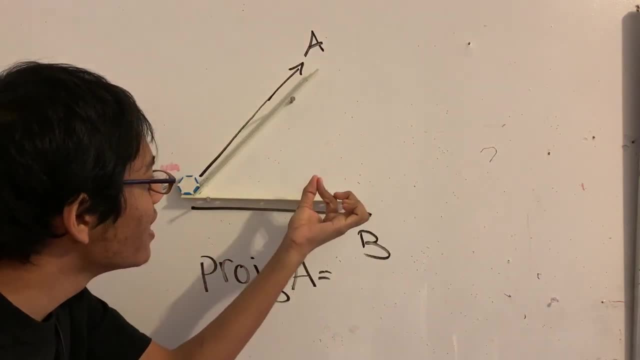 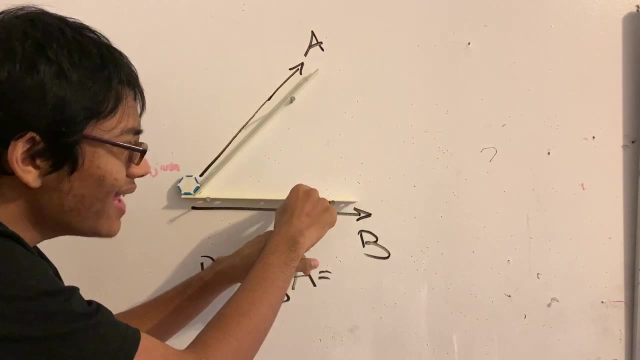 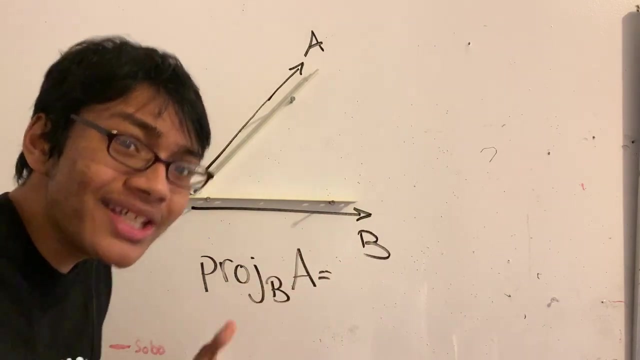 and it was shining down on vector a. Well, it would shine down in just the right way, so that a bit of the light would pop up here and that bit of the light would come back. light would be the shadow of this vector a onto vector b. so when we say projection, we're really 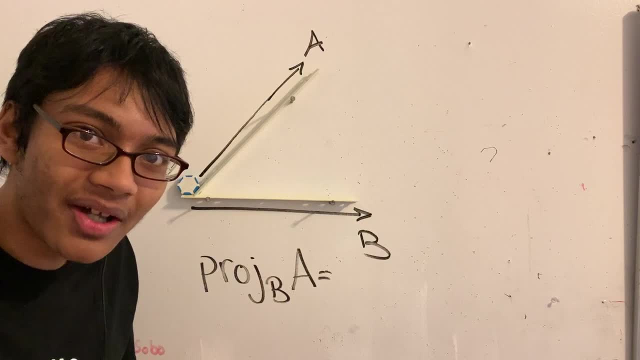 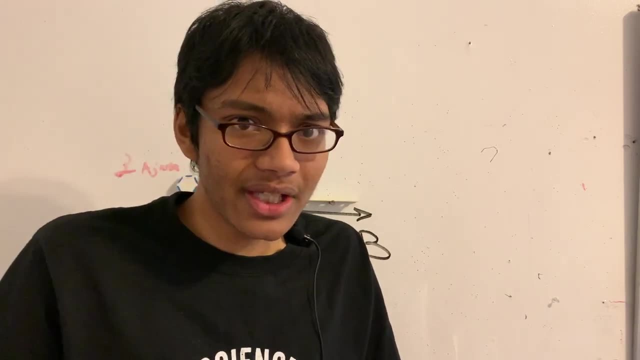 talking about shadows, but you don't have to think about it, you don't have to imagine it. here it is. this is a 100 milliwatt laser classified as a weapon here in the us, but today we're only using it for educational purposes, if i screw off the lid over here. 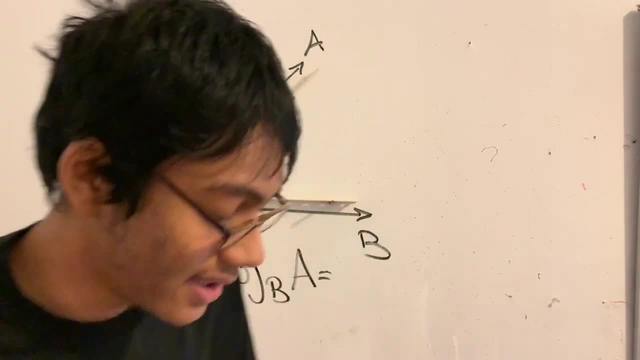 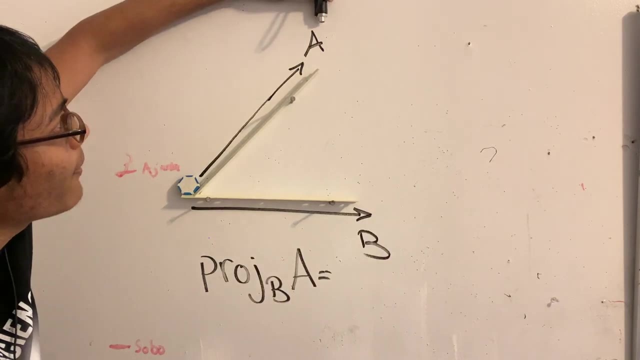 so that the light is not too focused, otherwise it would be blinding. then i can shine it from above, vector a, almost like a street lamp right, and what do you think is going to happen? what's going to happen? well, what's going to happen is the projection, the shadow of vector a is going. 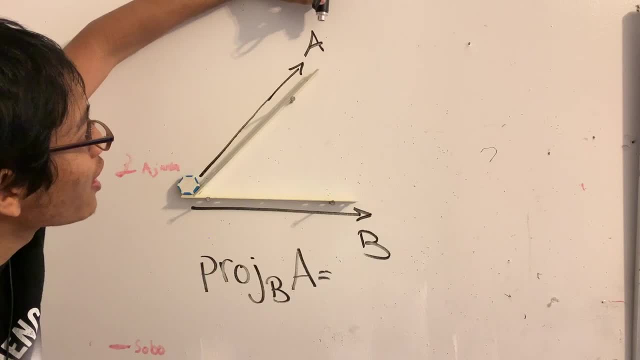 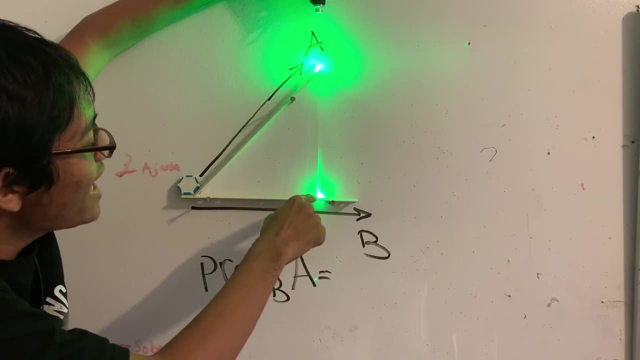 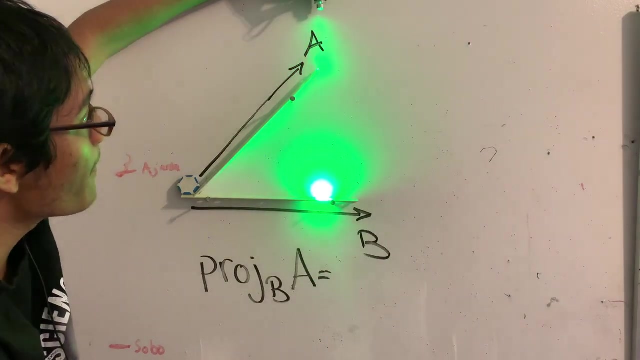 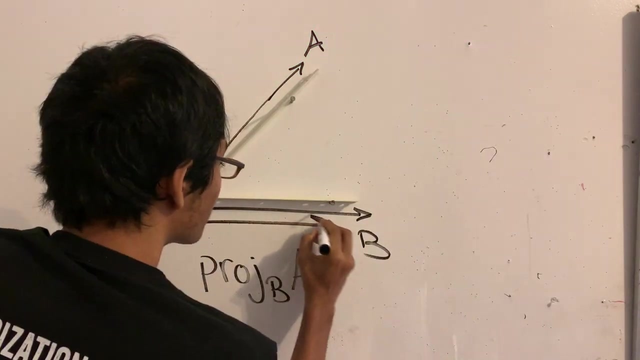 to pop up on vector b. let's check it out. enough talk and there you go. that right, there is the projection of vector a onto vector b. now look at that closely and you'll realize something of major importance. right, this projection of vector b is here. the projection of vector b is the projection of area a and the projection 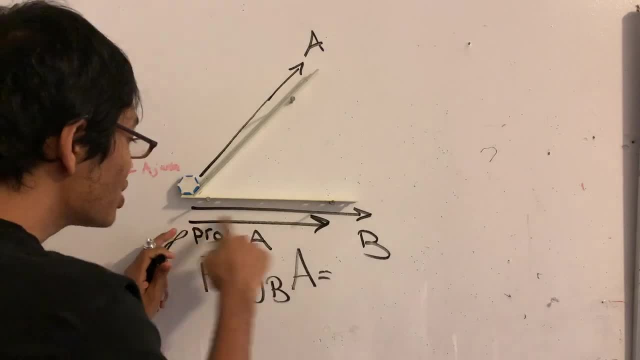 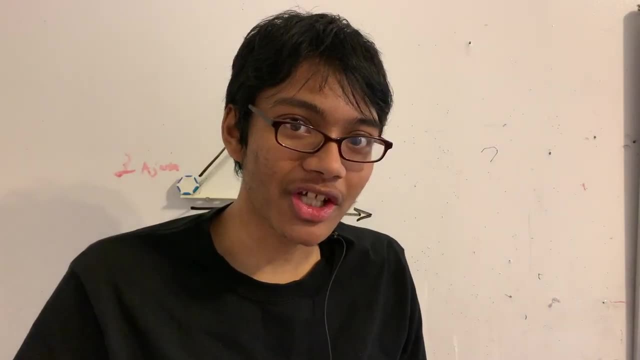 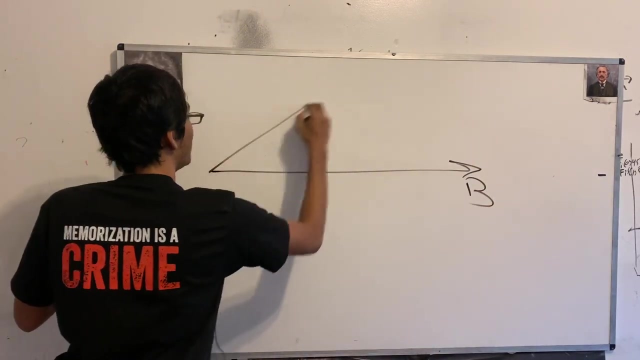 itself is a vector. that projection itself was a vector, right? this was the projection we were looking for, proj b a- and just like any vector, this projection has a magnitude and a direction. but how do we find that magnitude and direction? that's what we're gonna do, all right, so here's. 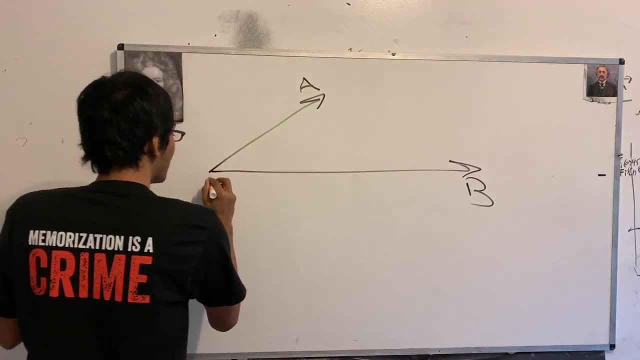 the deal. i got my vector b right here and my vector a right here. of course, i want to find the projection of my vector a on to b, which is going to look something like that. all right, so we're like this vector. this vector. let's call my projection vector u, just for the time being. 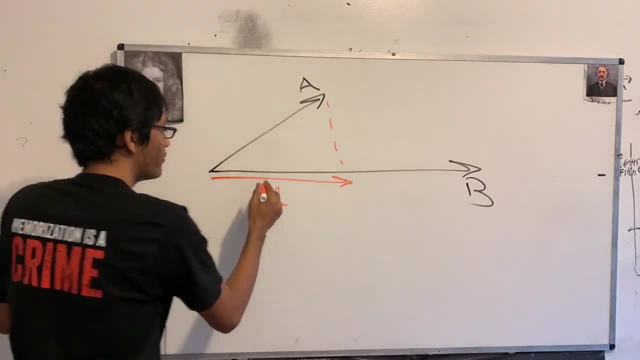 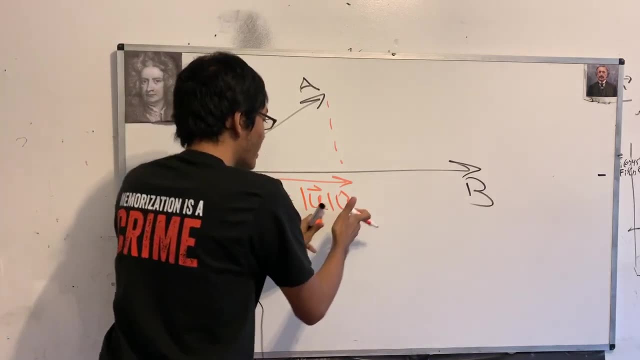 now, now. now now. how can we find this projection vector? well, like any vector, it's going to have some magnitude and some direction, right? so how do we find that magnitude and that direction? well, here's something you can use to your advantage: this theta here, this cosine theta. 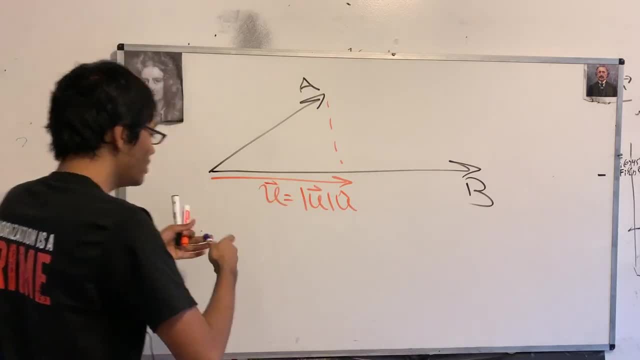 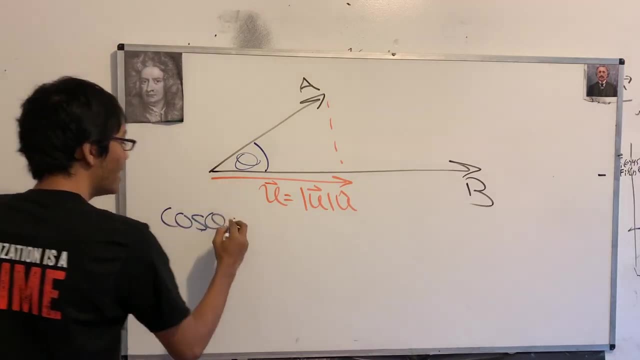 find that magnitude and that direction. well, here's something you can use to your advantage: this theta here, this cosine, theta right here, so we can say cosine of this angle, theta is going to be adjacent. what's that adjacent here? that's going to be the magnitude of u over what's my hypotenuse? well that's. 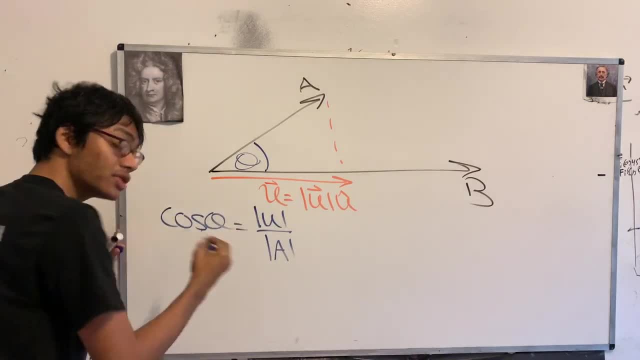 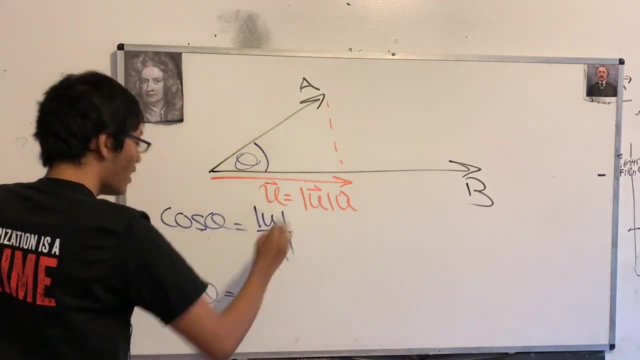 going to be a, that's going to be a. ladies and gentlemen, now we can also use the dot product cosine definition, which says that the cosine of theta is going to be the dot product of what, in what, of a and B over the magnitude of a times. 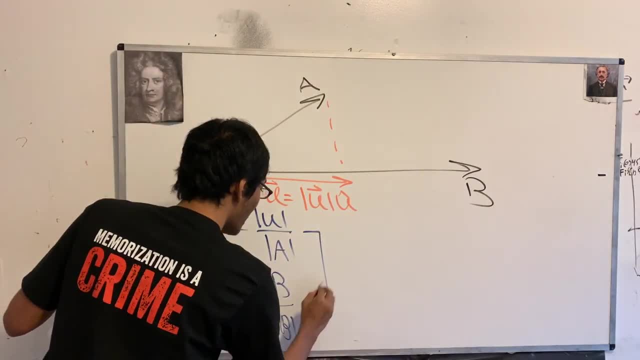 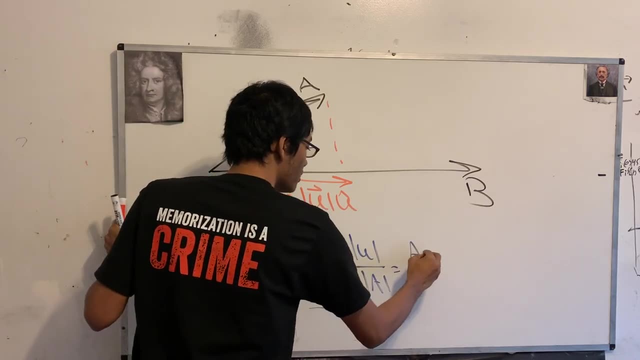 the magnitude of B. set these two things equal to each other. what do you get? what do you get? well, you're going to get. the magnitude of u over the magnitude of a is equal to a dot B over the magnitude of a times the magnitude of B, and we're almost there. 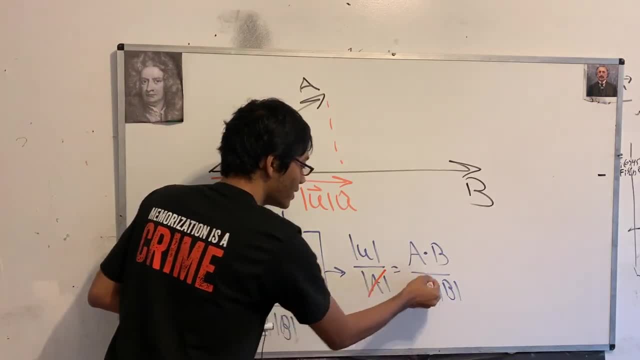 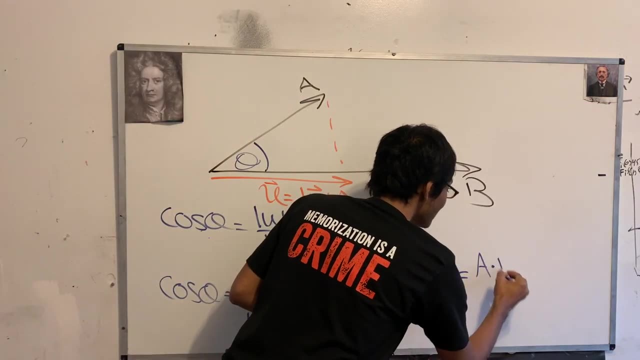 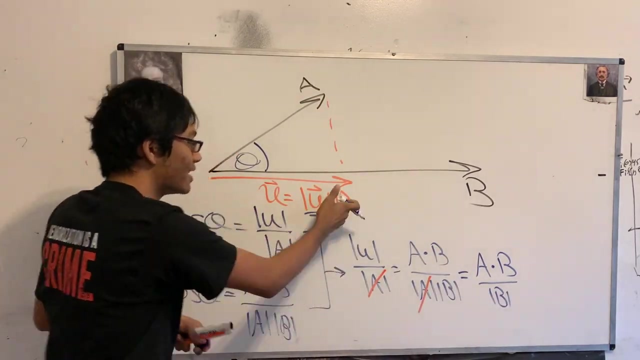 ladies and gentlemen, we're almost there. these two guys drop out, cancel out and we're left with the magnitude of u, which is a dot B over the magnitude of B, but we still need. we have the magnitude, but we still need the direction. we have this part, we still need this part. the 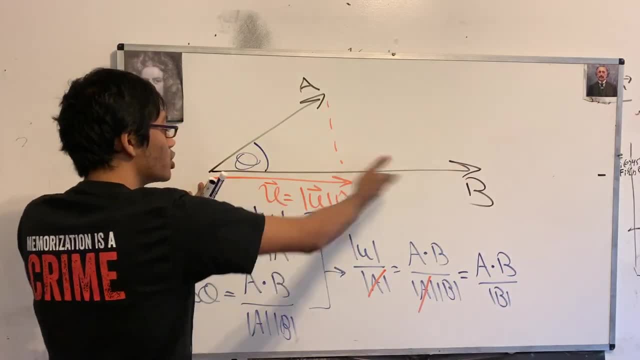 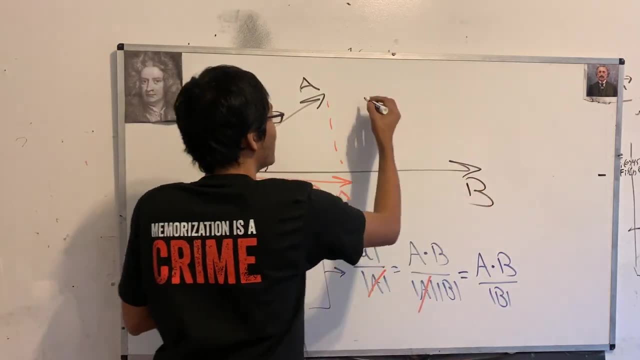 direction. now notice, the direction of our, of our projection is going to be in the same direction as this vector B that we're projecting onto. and what's the direction of vector B? well, it's going to be the unit vector right. what's the unit vector for B? well, it's going to. 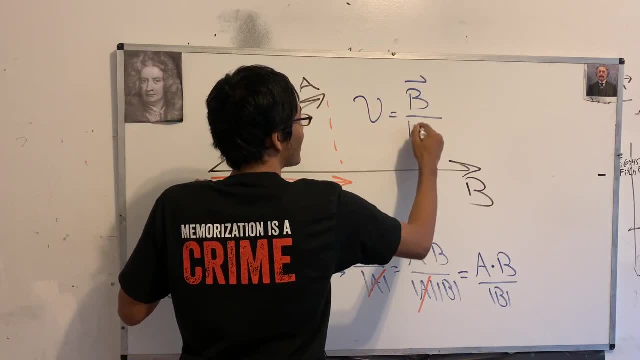 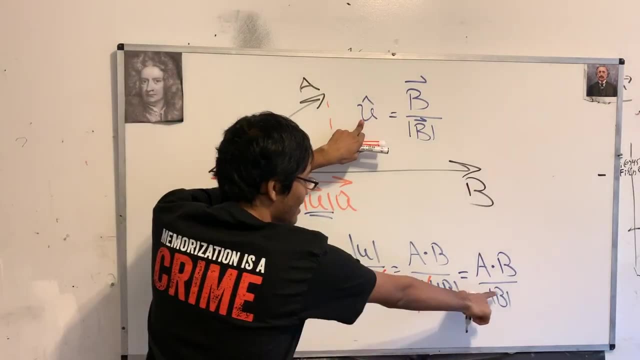 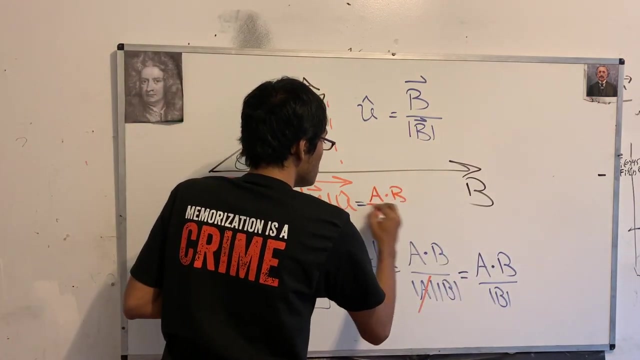 be the magnitude of B, or rather B itself over the magnitude of B. and so now, if we go ahead and multiply these two guys together, the direction and the magnitude, we're going to get our final, our final projection. so that's going to be a dot B, a dot B over the magnitude of B times B over the. 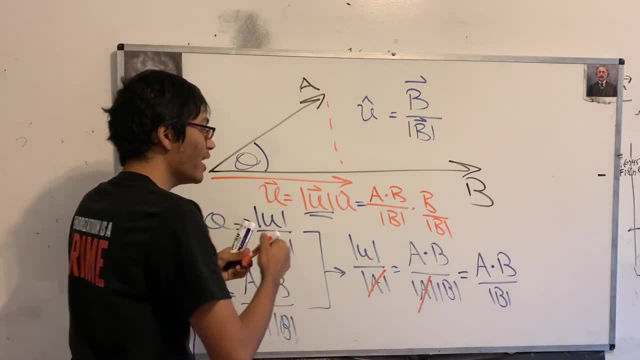 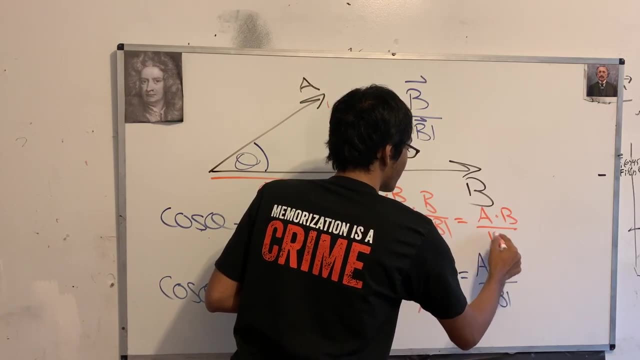 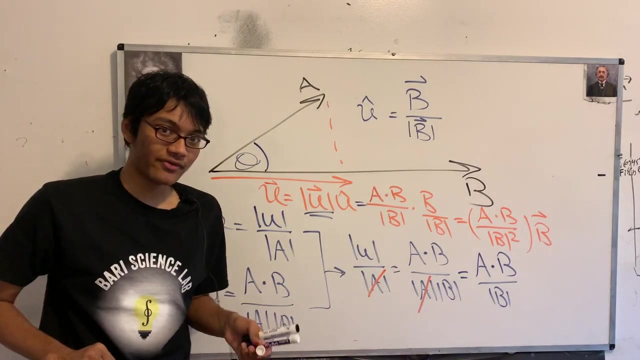 magnitude of B, ladies and gentlemen, and we're almost there. so what is this going to simplify? to? well, we're going to have a dot B on the top, divided by the magnitude of B, squared all times B, and that, right there, ladies and gentlemen, is the projection formula. thanks for watching, and we'll check you out in the next episode of vector calculus. 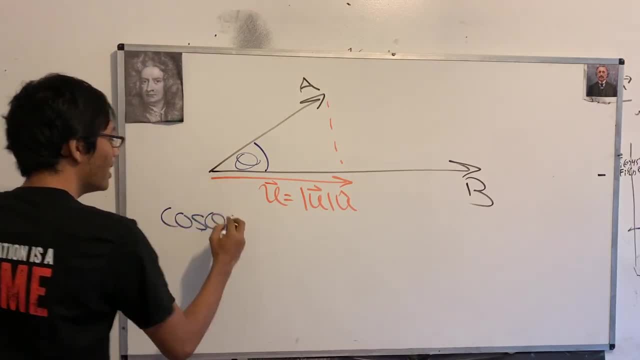 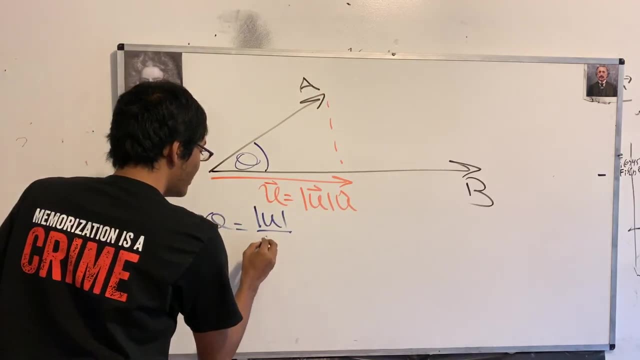 right here, so we can say: cosine of this angled theta is going to be adjacent. what's that adjacent here? that's going to be the magnitude of u over what's my hypotenuse? well, that's going to be a, that's going to be a. ladies and gentlemen, now we can also use the dot product cosine definition. 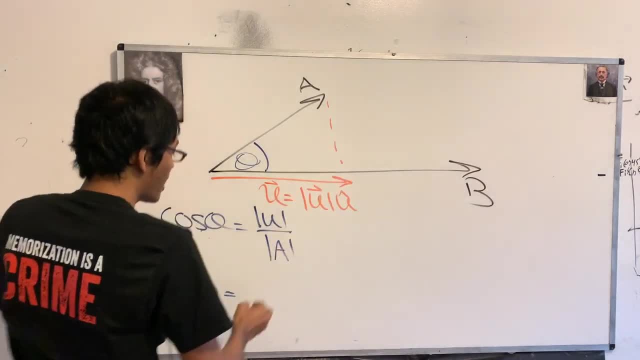 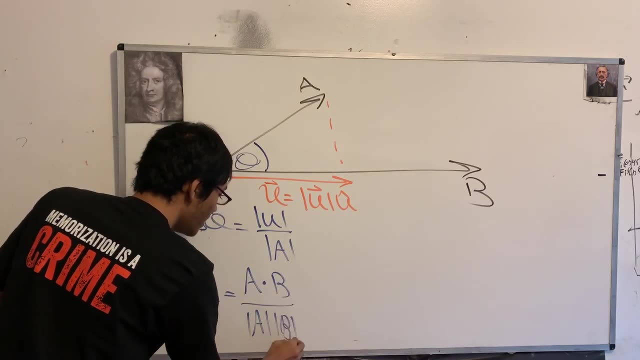 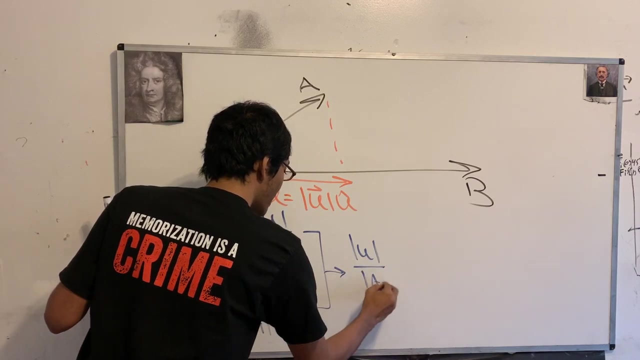 which says that the cosine of theta is going to be the dot product of what and what of a and b over the magnitude of a times the magnitude of b. set these two things equal to each other. what do you get? what do you get? well, you're going to get the magnitude of u over the magnitude of a. is 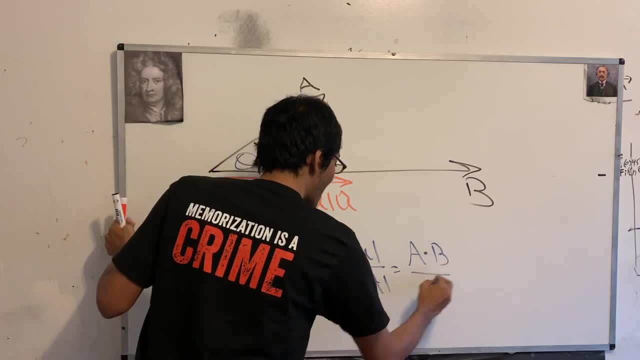 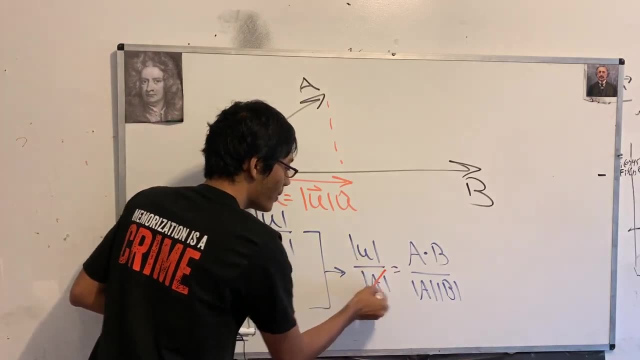 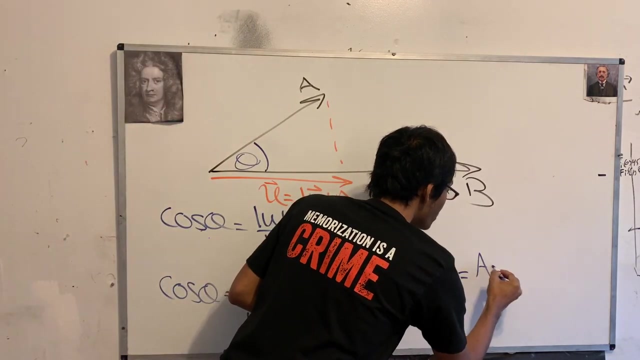 equal to a dot b you, over the magnitude of a times the magnitude of b. and we're almost there, ladies and gentlemen, we're almost there. these two guys drop out, they cancel out, and so we're left with the magnitude of u, which is a dot b over the magnitude of b, but we still need, we have the magnitude, but we still 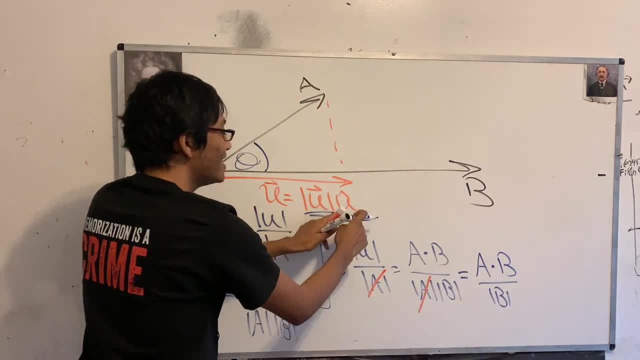 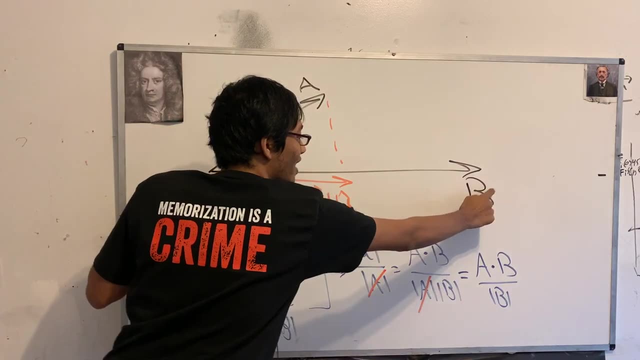 need the direction. we have this part, we still need this part. the direction, now notice, the direction of our, of our projection, is going to be in the same direction as this vector b that we're projecting onto. and what's the direction of vector b? well, it's going to be the unit vector. 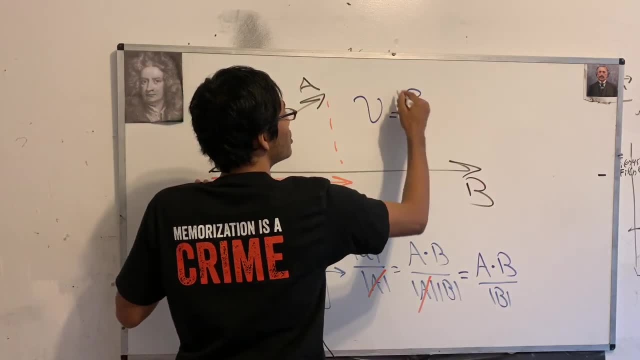 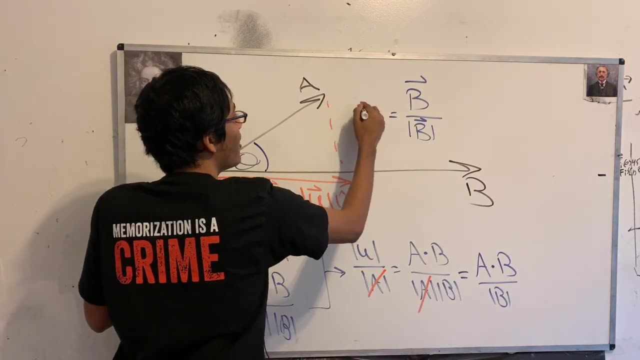 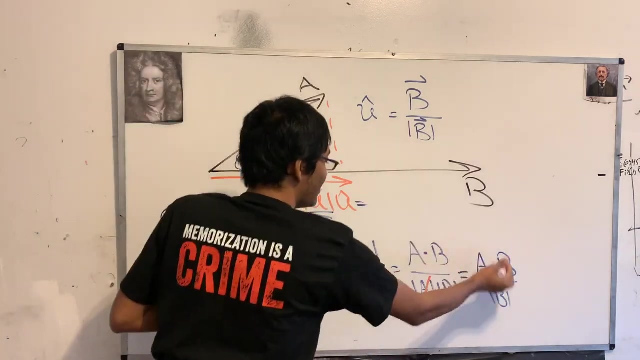 right, what's the unit vector for b? well, it's going to be the magnitude of b, or rather b itself over the magnitude of b. and so now, if we go ahead and multiply these two guys together, the direction and the magnitude, we're going to get our final, our final projection. so that's going to be a dot b. 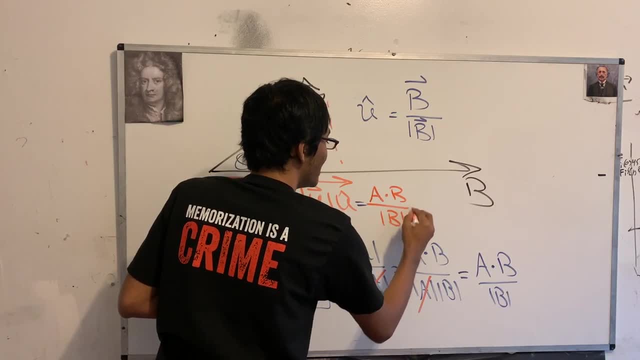 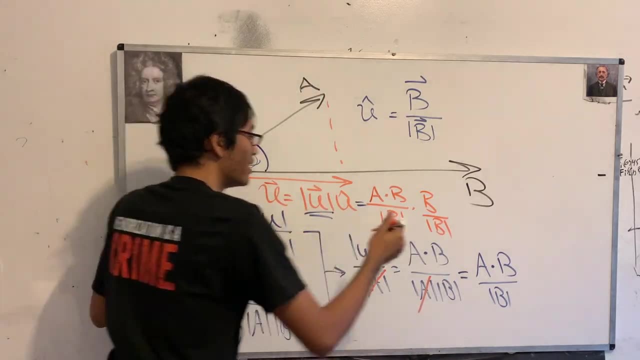 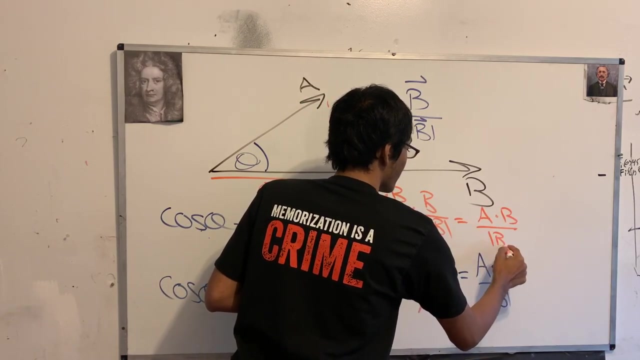 a dot b over the magnitude of b, times b over the magnitude of b, ladies and gentlemen, and we're almost there. so what is this going to simplify? to well, we're going to have a dot b on the top, divided by the magnitude of b, squared all times b, and that, right there, ladies and gentlemen, is the. 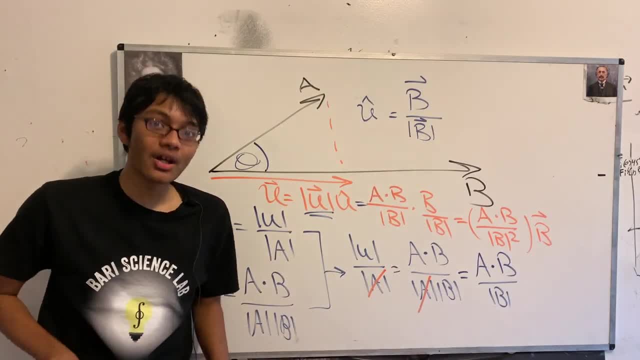 projection formula. thanks for watching and we'll check you out in the next episode of vector calculus. you.